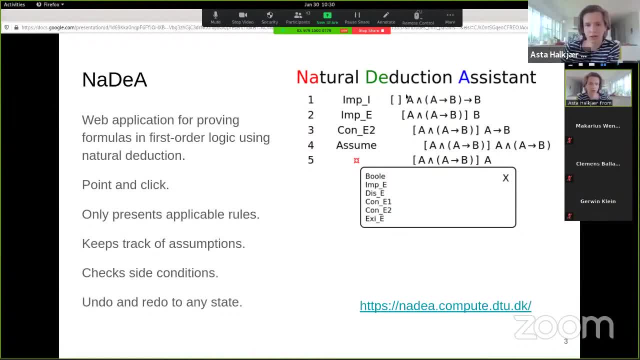 And so you can see a screenshot of part of it over here on the right. What you do is you input a formula using point and click, And then the system will give you this little red sun which tells you applicable rules for proving this formula. 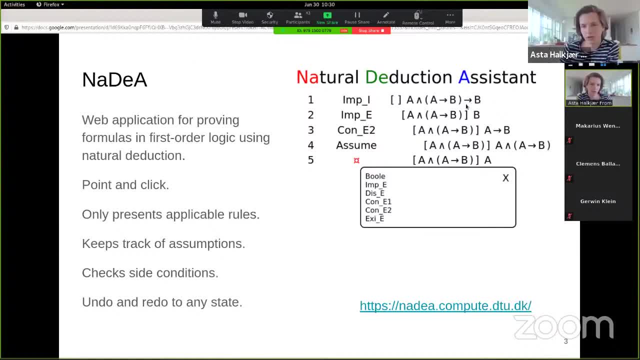 So on the first line, you see, the outermost operator is an implication And we've chosen to try to prove this with an implication introduction. So the conjunction moves into the list of assumptions And now we're asked to prove B. Then we can continue this proof like that. 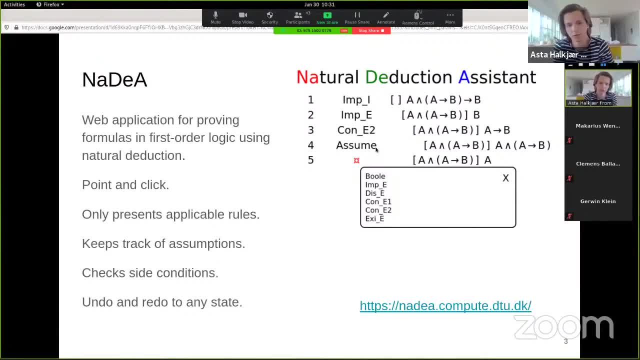 And the system does a number of nice things for us. It only presents applicable rules, So the student is not overwhelmed by a complete list of rules every time. It keeps track of assumptions. So this line 4 is automatically discharged when we input this formula. 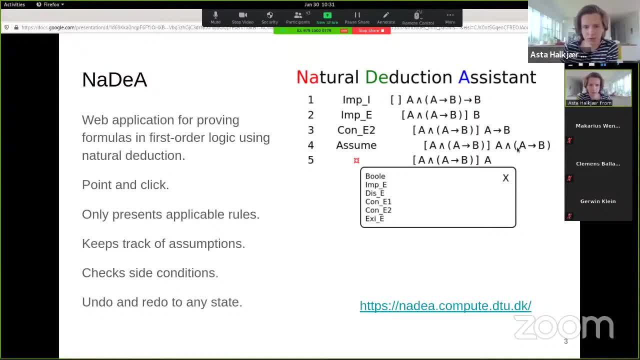 It checks side conditions of the rules. This is full first order logic And it also supports undoing and redoing to any state. So you can undo something, do a few things, undo those things and then redo to where you were at the beginning. 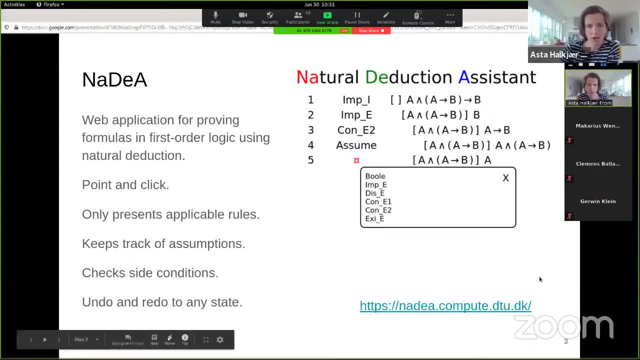 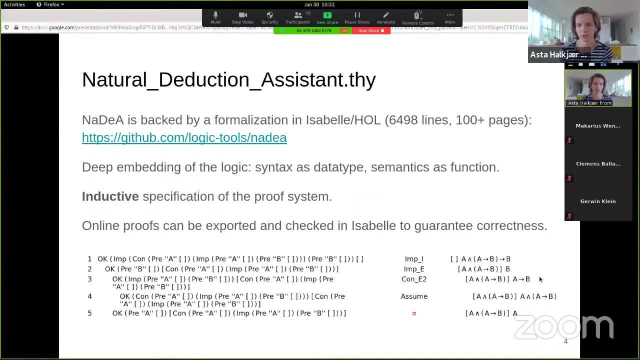 And it's available on this address Now. so what sets our system apart is that it's backed by formalization in Isabel, which is more than 6,000 lines, And it's available on GitHub. So it's a standard deep embedding of the logic. 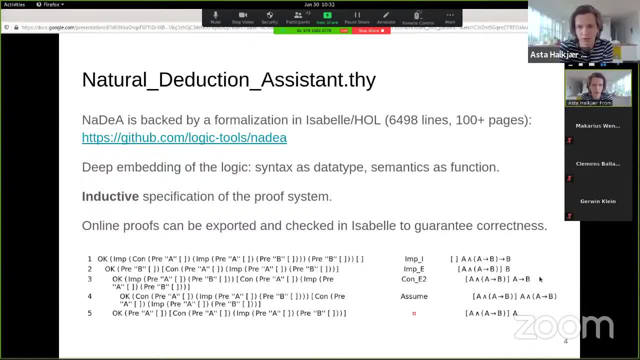 We have the syntax as a data type, We have the semantics as a function on this data type. Then we have an inductive specification of the proof system And, even though the online application is not formally verified, we can export proofs. Then you can check them in Isabel. 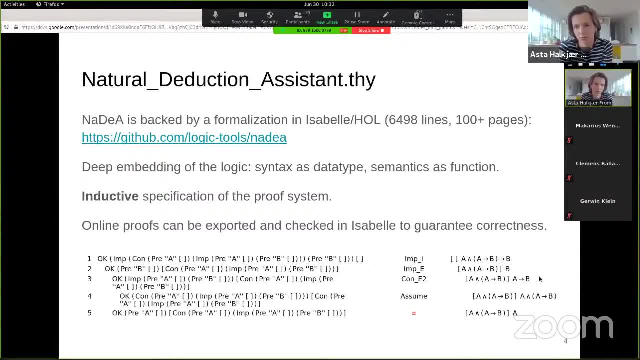 export it to Isar notation And the formalized soundness proof will guarantee the correctness. Another feature of the online application is that you can see the abstract syntax. You can. this is if you can click on click the application, it will go into this view. 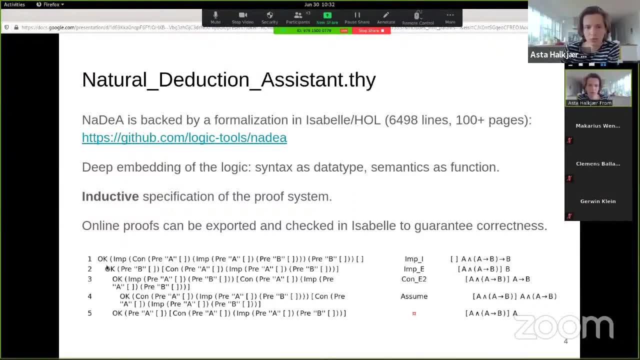 where you see this inductive predicate. okay, which is the proof system? The first argument is the formula you're proving And the second argument is the list of assumptions, And so this will familiarize students with this data type construction of formulas. So, just to briefly introduce, so, syntax and semantics. 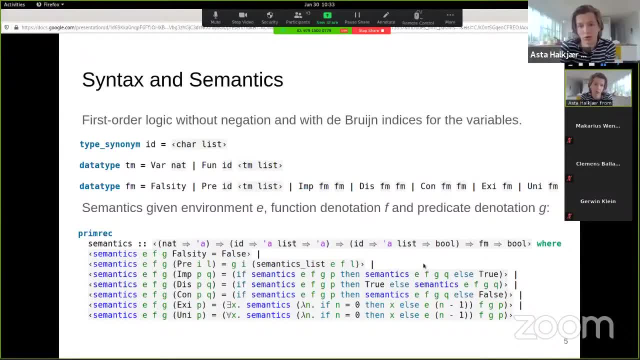 or it's first order logic without negation. We use the point indices for the variables. Our identifiers are just strings And we have, so we don't have negation, but otherwise we have the usual connectives and both quantifiers. The semantics are as you expected. 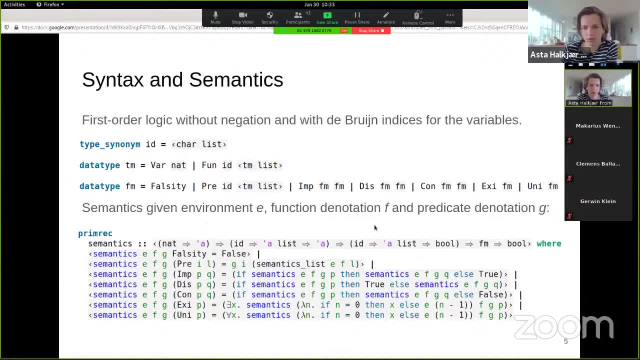 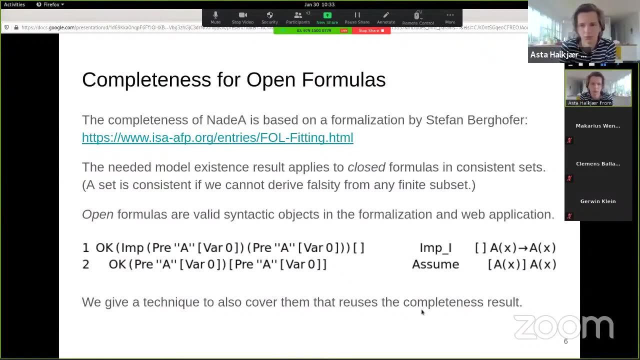 We expect them to be given an environment, a function denotation and a predicate denotation And you can see the quantifier cases. There's some shifting of variables to do with the point indices. So the completeness, so this system is proof, sound and complete. 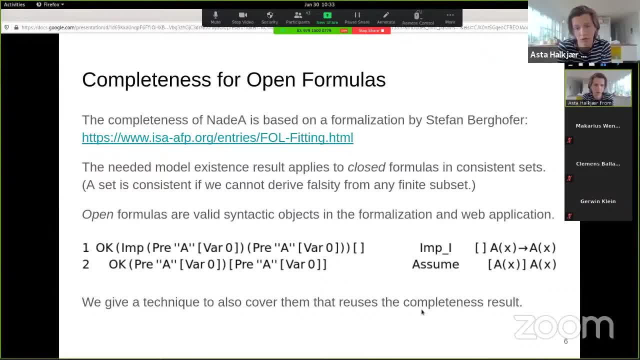 The completeness is based on the formalization by Stephen Backhofer of Fittings work, And there the model existence results. it applies only to close formulas. But then I ask. so I did this work for my bachelor thesis and I thought: what about open formulas? 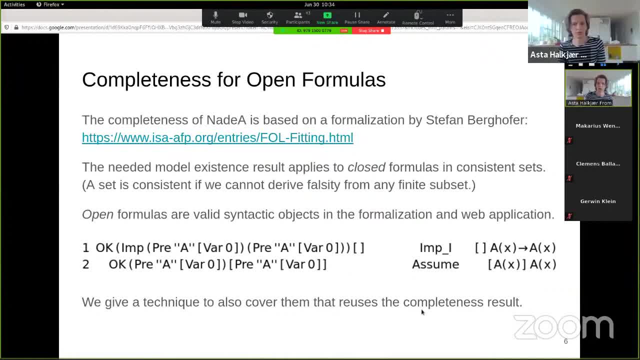 They are valid syntactic objects in both the formalization and the web application. So can we be sure that a proof exists for an open formula? Here's an example. You can just so. if you put in zero as a deployment index, you don't have any quantifier. 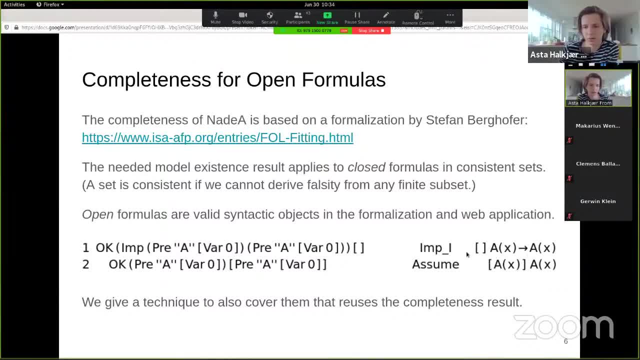 then you get an open formula. This is how it would look in the web application also, And so I wanna spend the second part of the talk just talking about a way to reuse this completeness result to cover for closed formulas, to also cover open formulas. 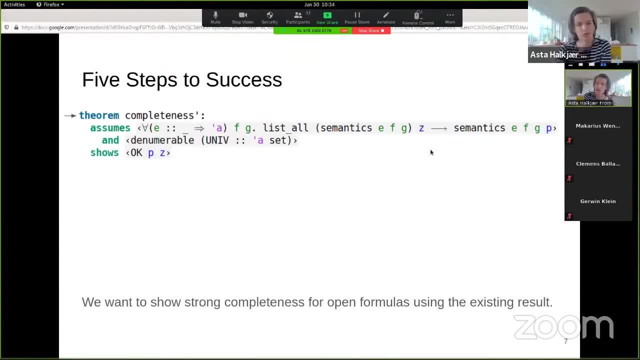 There are five steps to success. So what is the context here? The context is that we want to show you, we want to show strong completeness for open formulas using the existing result. So we assume that under the assumption set, this formula P holds. 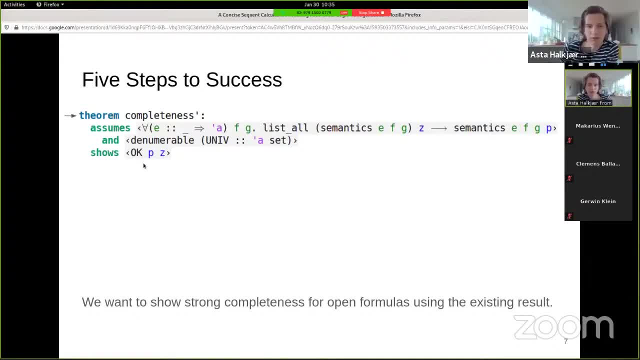 And we want to show that there is a derivation of P from assumption set. So what do we do as a step one? Well, we take these assumptions and we build a chain of implications In the object, on the object level. So, instead of having this meta-learn notion of assumptions, 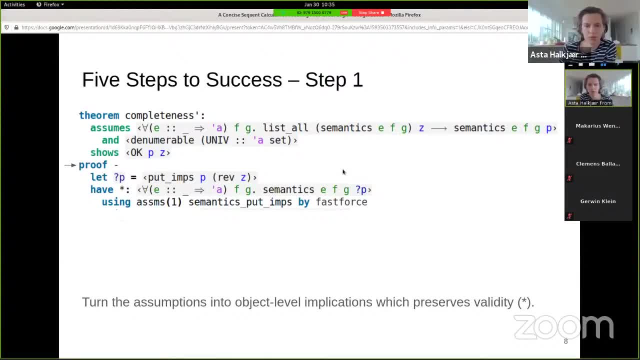 we just build a formula which is a bunch of implications changed after one another, And we call this question mark P, And it's easy to see that this formula is invalid based on our assumption. Then we close the formula with the universal quantifiers. 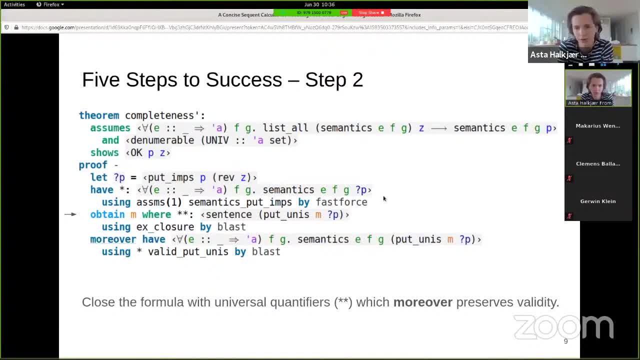 If you just add a sufficient number of them, that will close the formula And this also preserves validity. And now we have a closed formula. So now our completeness result for sentences applies and we can get this derivation of the universal closure of the formula. 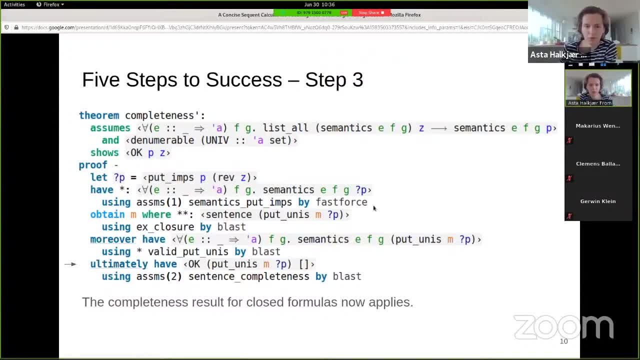 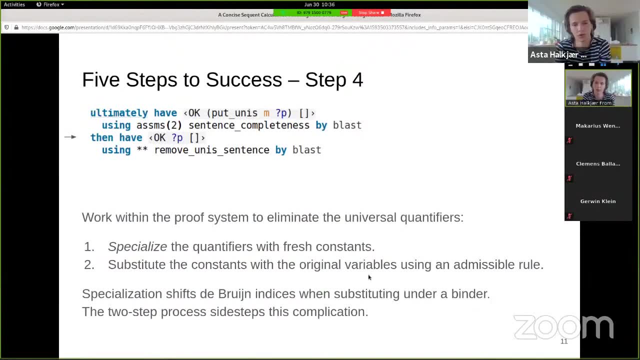 built from implications and from the empty list of assumptions. So now we move to working within the proof system. So we want to do two things: We want to first eliminate the quantifiers again and we want to turn the implications back into assumptions. 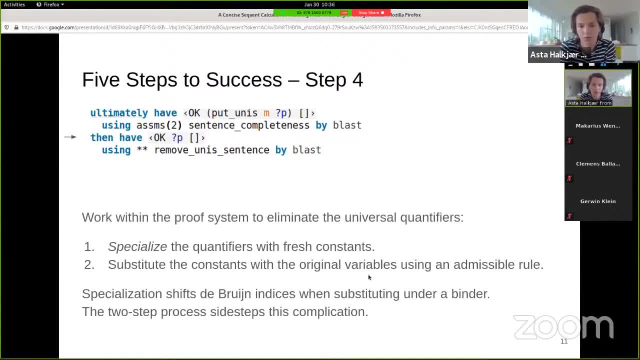 So, to eliminate the quantifiers, we specialize them with fresh constants and then we substitute these constants with the original variables using an admissible rule, And so, yeah, we have a very simple, pretty simple. you may wonder why not just specialize directly? 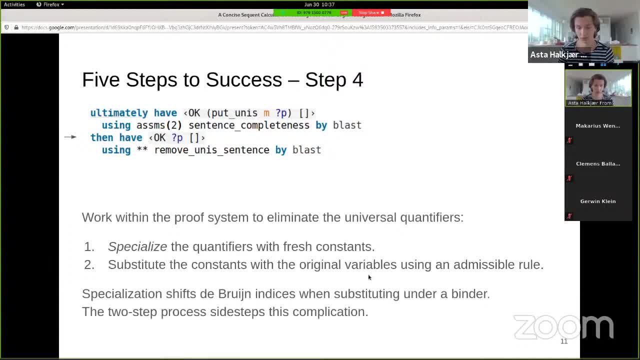 with the original variables. Well, we're using the point indices. I'll get into this more in the next slide. A specialization shifts the point indices when we substitute under a binder, And this complicates the reasoning we have to do, but doing it in two steps it sidesteps this complication. 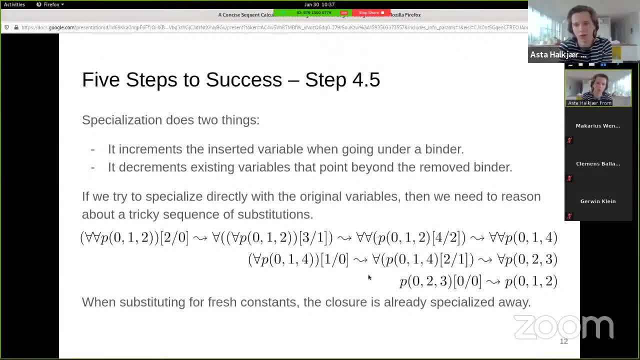 So again, so what happens when you specialize? I mean so you remove a quantifier, you insert some term instead of the quantified variable. So but then when you go, if we are inserting a variable, specializing with a variable, 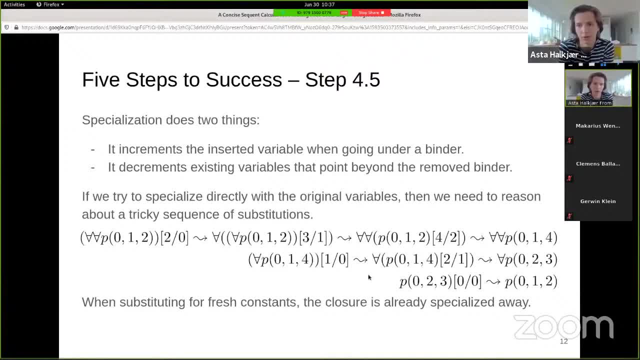 then you have to increment this variable when you go under a binder, because now it's pointing, it needs to point at the same thing, but now you went under binders. you have to account for that And, moreover, specialization removes a quantifier. 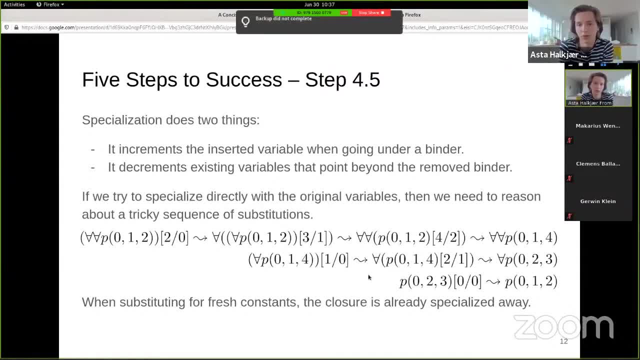 So you have to increment every existing variable that pointed beyond the removed binder. So let's look at this chain of substitutions. So let's say we have this term P with variables zero, one and two. It had originally three quantifiers in front of it. 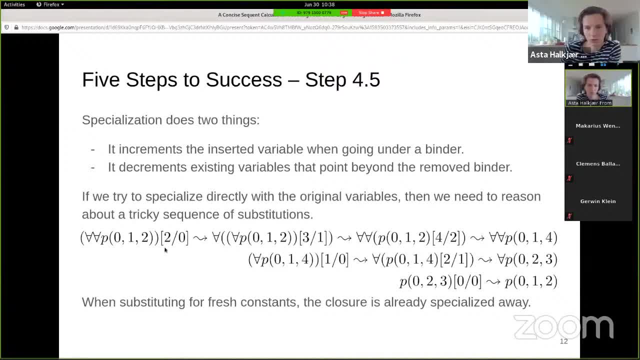 And now we are specializing the first one with a variable two. So when the substitution goes under the first binder, we are now substituting three for one, Then we're substituting four for two, And so the resulting term after this first substitution is zero: one four. 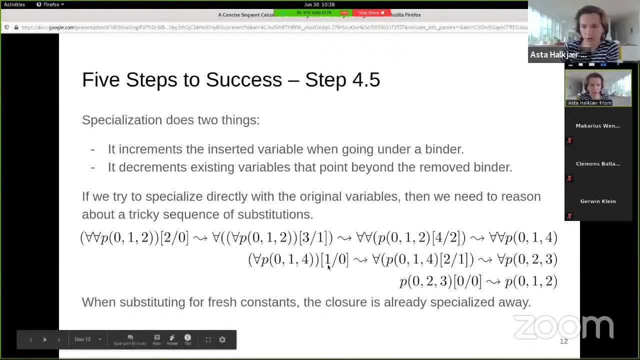 Similarly, when we specialize the second quantifier with the variable one, the resulting term becomes zero, two, three. And only when we specialize away the very final introduced quantifier do we get the variables that we actually want. And so, biographically, this happens here. 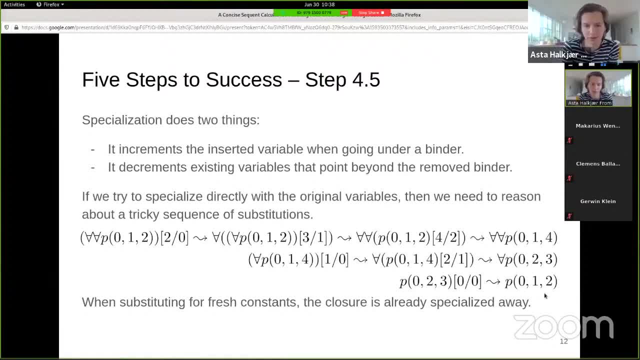 So there, this can be through dividing by select two, one up, And so I tried to think about this and it was too tricky for me. So instead we specialize with constants, which is just: these are not incremented when you go under the binder, so there's no trouble there. 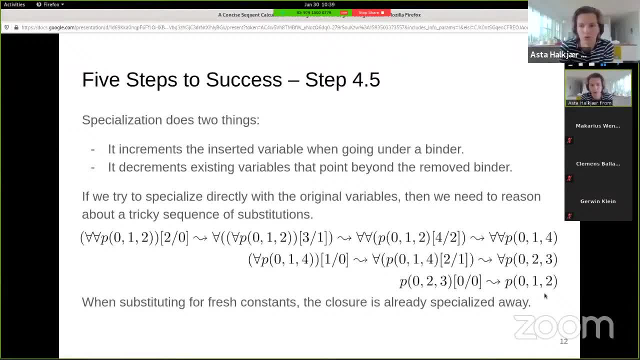 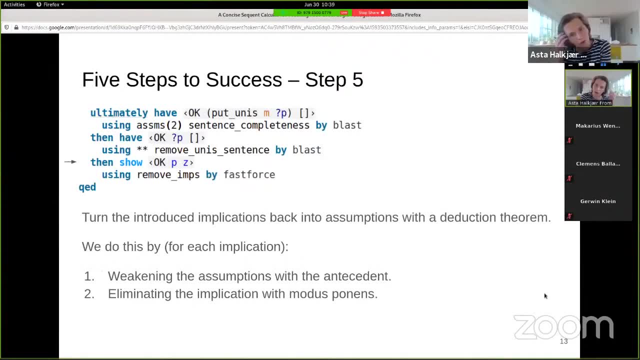 And then when you substitute the constants with the original variables, then the closure is already specialized away. So we start set this complication. So when we go back to step five, we just need to turn the introduced implications back into these meta-assumptions and it's basically the deductions theorem. 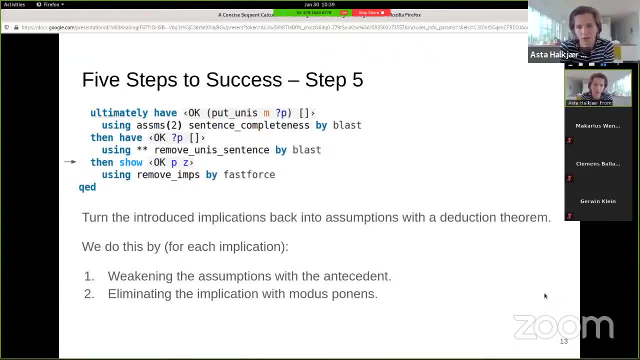 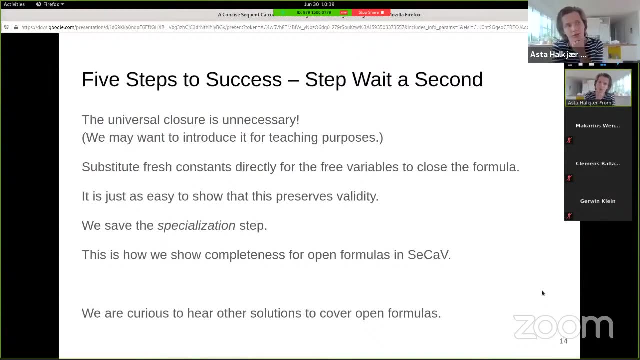 So what we do is we weaken the assumptions with the antecedent and then we eliminate the implication with modus ponens, and we just do this for each implication And step away. Let's see Second. so we did something unnecessary here. 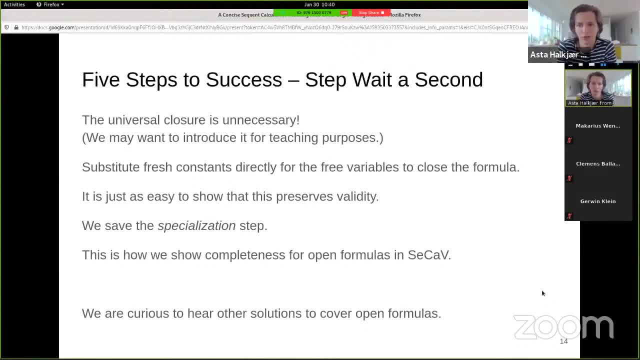 So we introduced the universal closure, got the proof and then immediately specialized it away. But why don't we just substitute the fresh constants directly for the free variables and close the formula this way? So maybe we want to introduce the universal closure for teaching purposes, but we can. 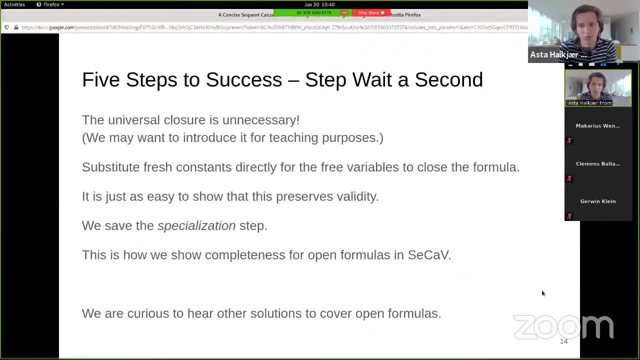 save the specialization step if we close the formula by substituting open variables with fresh constants, Free variables and fresh constants instead of adding quantifiers. And this is how we have done it for the SQL calculus. But it's still, even if it's four or five steps, it's a bunch of steps to do this. 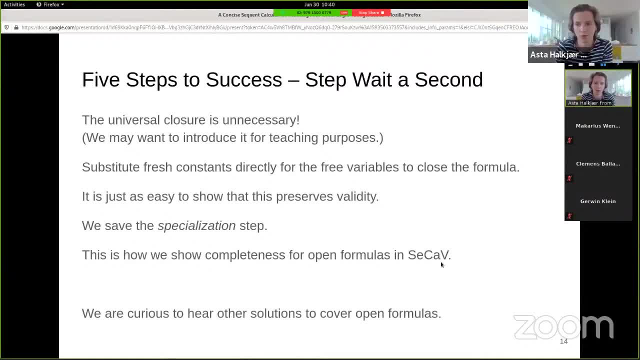 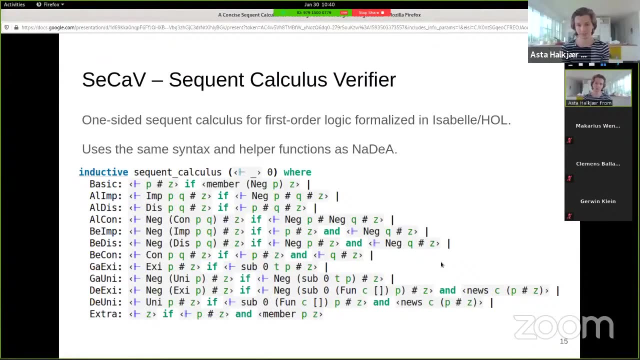 So we are curious to hear other solutions to cover open formulas that are not just universally. closed them and consider them the same. Then we reach the end of the session. So we have reached the SQL calculus third part of the talk. So what is it? 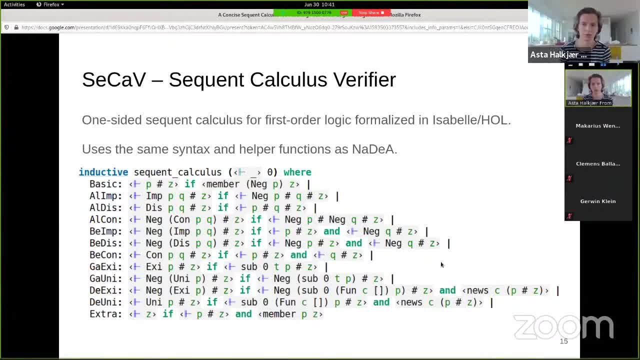 It's a one-sided SQL calculus that we introduce after they have seen the natural deduction. It's the same syntax and helper functions as Nadea And it's designed to just be as concise and simple as possible, while covering the full syntax and the full logic. 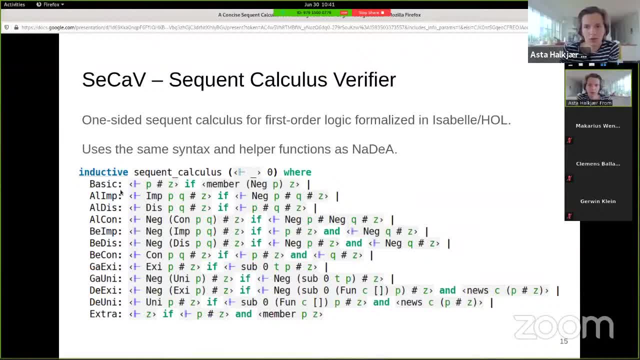 So we have these basics, Basic sequence, which, if you have a formula at the very front and it occurs negated somewhere in the tail, then this is a sequence that you can derive And then every rule works on the first and the head of the list of the sequence. 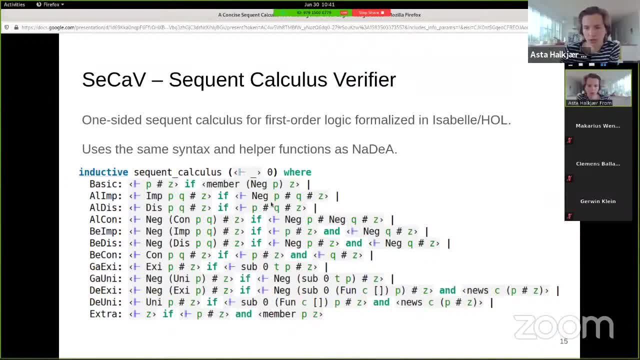 So, for instance, an implication is broken down into a negated antecedent and the consequent, and so on. The rules follow Smulyan's uniform notation. So we have alpha rules, which are propositional and do not branch. We have beta rules, which are propositional but do branch. 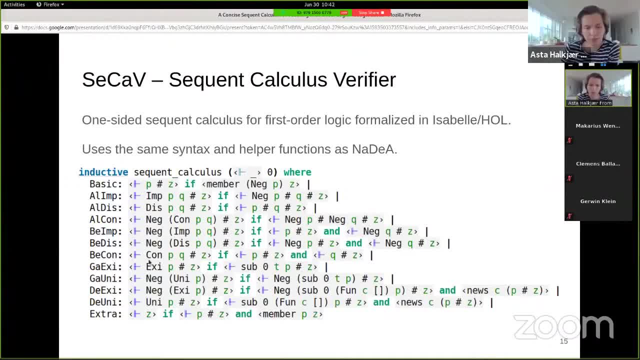 So now we have two sub-derivations we need to do. The gamma rules apply to every instance So we can build an existential for any witness, But the delta rules they. I mean, if you're going to introduce a universal quantify, then the instance you are abstracting. 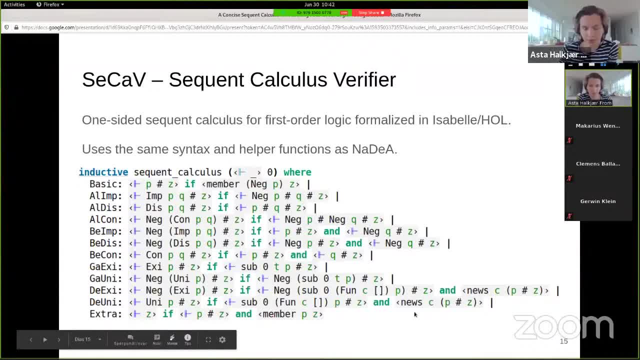 over it. better be arbitrary. But the students, they know these definitions from Nadia already. And then we have the structural rule extra, which says that if you have a formula at the head of the list and you can prove this sequence, but this formula is actually a member of the 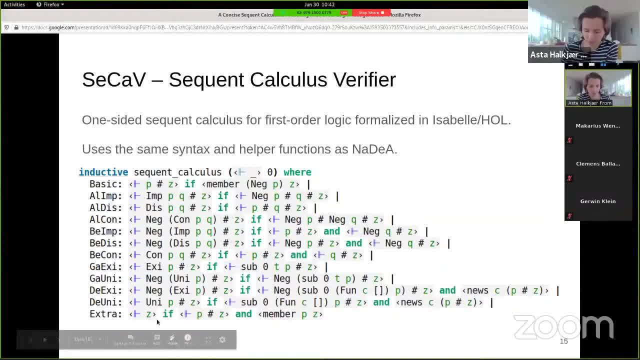 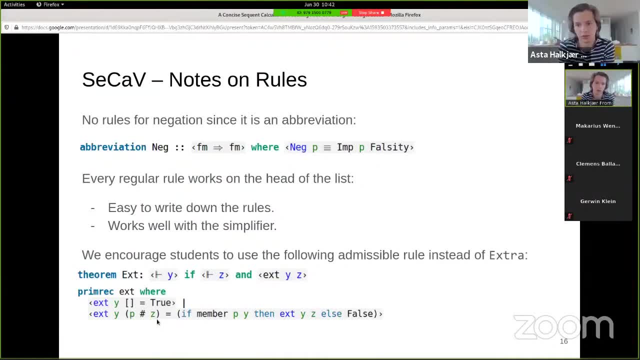 tail, then you don't need it at the head. So we have no rules. The rules for negation, because it's the same syntax as in Nadia. so it's an abbreviation, It's covered by the implication rules And every regular rule. as I said, they work on the head of the list. 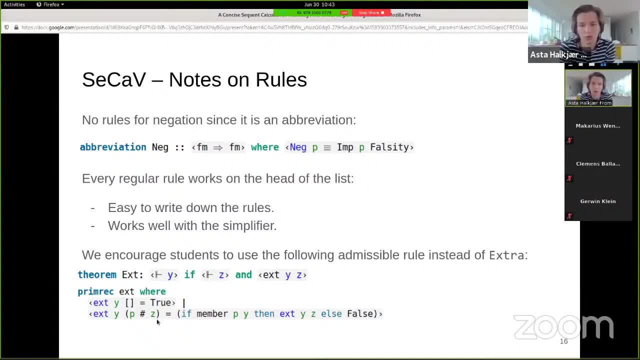 This makes it easy to write down the rules. It also works well with the simplifier, as we will see, And then the extra rule is a bit tricky to work with, as you can imagine. So we encourage them to use this extra rule. 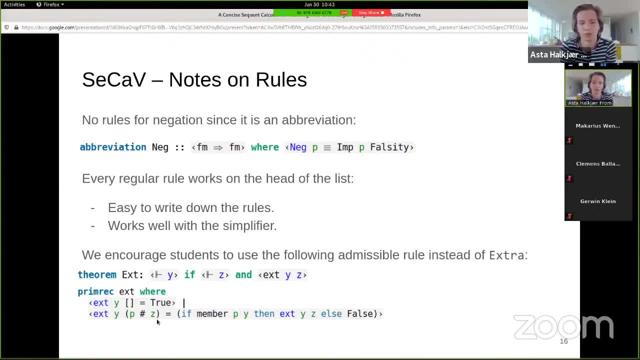 You know this ext rule Instead, which is admissible. it just says that you can prove, you can prove set and you can prove any extension, which just means that it has at least the same formulas, But they may be in a different order, they may be contracted or duplicated. 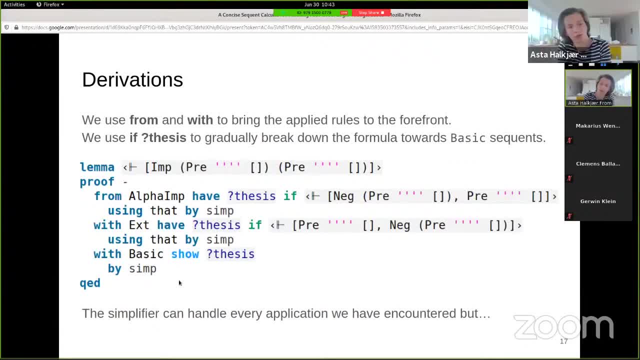 So in the course we use this template for writing down derivations where we used from the left side, and then we use the same rule with to bring the applied rules to the forefront, So you can read the left side and see exactly what rule is applied for each step. 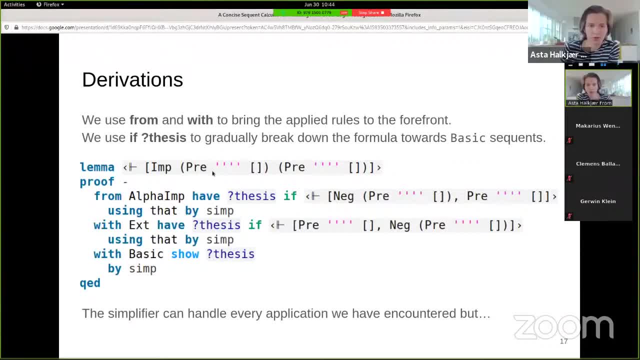 And then, instead of going so, we want to break down the formula instead of guessing the axioms and building towards it. So we use this if thesis, or thesis if construct to do that. And the simplifier, The simplifier can handle every application we've encountered. 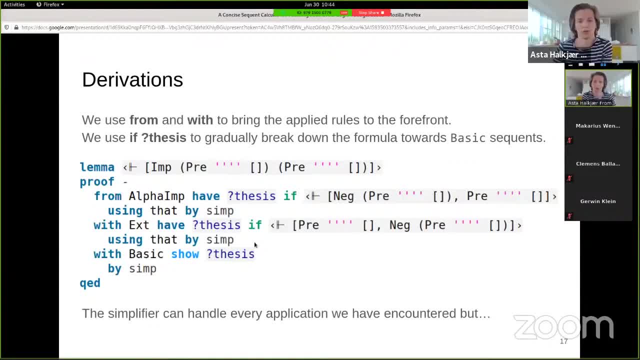 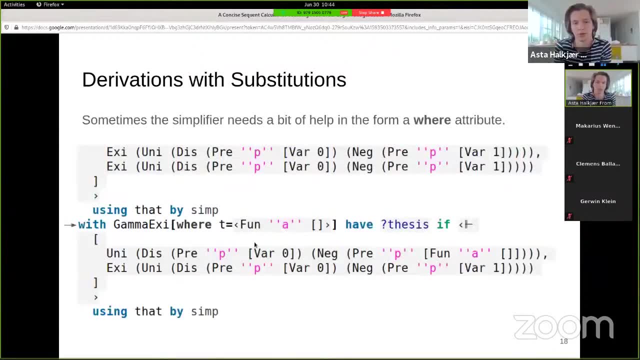 This is a very nice fallout of our specification, but sometimes, when there are substitutions, it needs a bit of help in the form of a where attribute. So we are trying to prove this existential. We want to prove it from this witness down here. 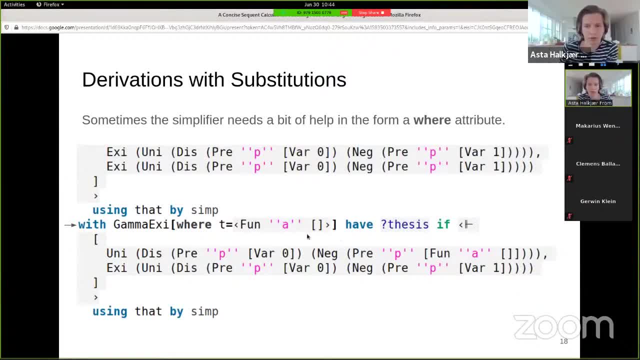 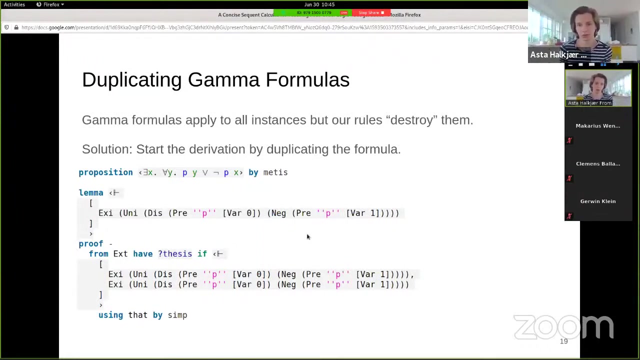 But if we admit the where attribute, Then none of the tri-zero approvers will find out, find this proof, And that is an unfortunate complication, but one that is fairly simple to work around. So the final thing, Gamma formulas. they apply to all instances, as I said, but our rules 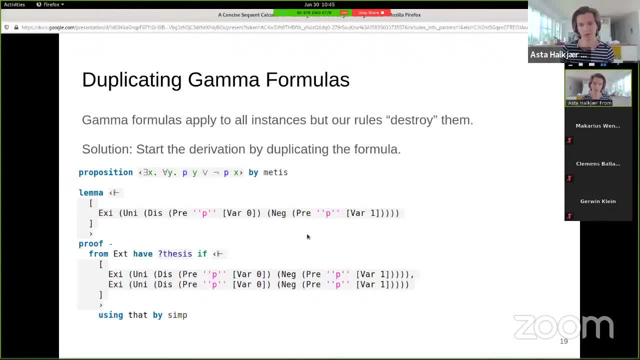 they destroy them. So the solution is to start a derivation by duplicating the formula. So the solution is to start a derivation by duplicating the formula. So the solution is to start a derivation by duplicating the formula. So let's say we're trying to prove this version of the drink as paradox. 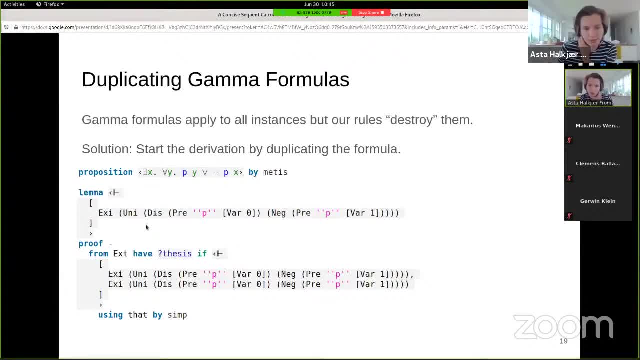 What we will find when doing the proof is that we actually need- we actually need to- to apply rule twice to this formula. So we start the derivation off by by simply duplicating it, Or, if you view it in the other way, 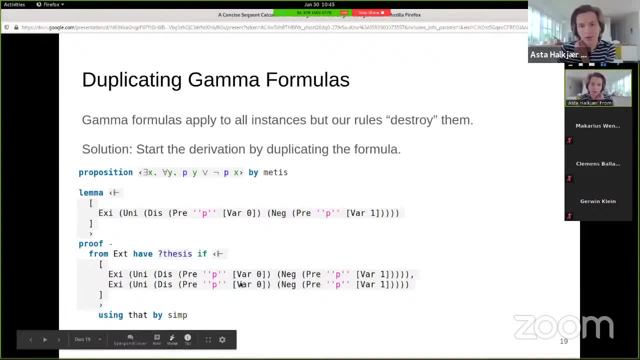 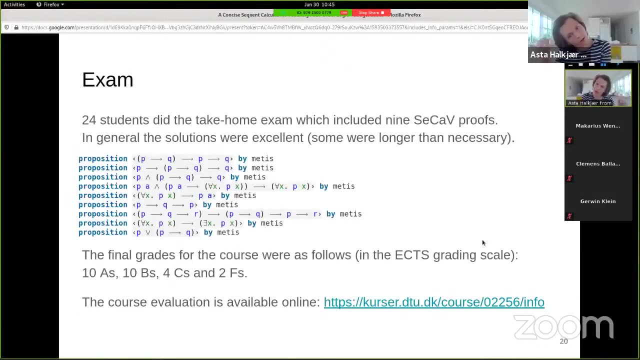 we enter derivation by contracting it And this is so in some textbooks. you see, like rules that you have to to keep the formula around And this, this is how we deal with this. So there was an exam in the course: 24 students. 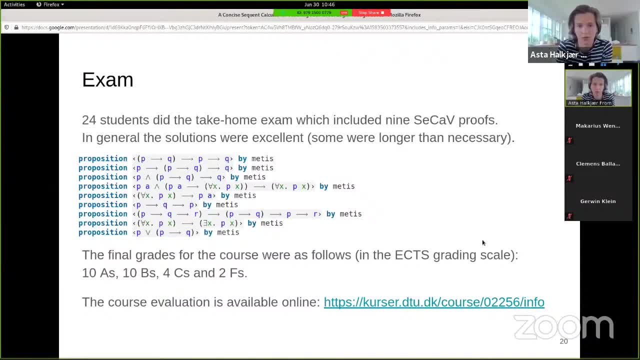 did the take home exam. There were nine proofs in this system Where they write: we give them a formula like this and they write it in Isabelle, And in general the solutions were excellent. Some proofs were a little longer than necessary, but but most of them. 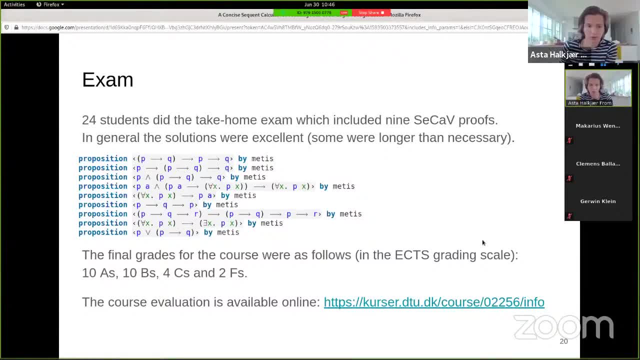 did excellent work. The final grades were also very good: 10 A's, 10 B's, 4 C's and then there were 2 F's, And you can see the course evaluation online if you want to, And that's actually serves. 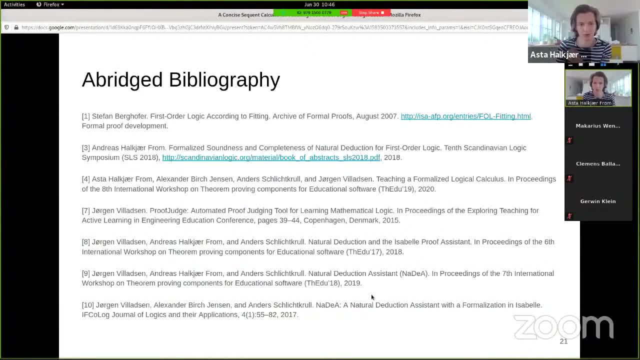 as my conclusion slide. So that's an abridged bibliography. You can see the full one in the paper, but these are the ones that pertain particularly to this, this presentation. So yeah, thank you for listening, Thank you for your talk and the floor is open. 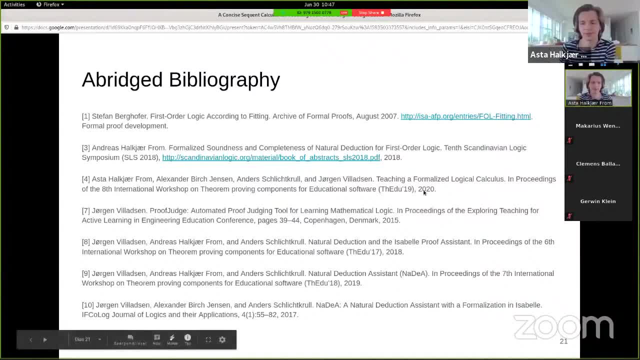 for questions. Dimitri seems to have a question now. Dimitri is applauding. Am I supposed to do something? No, I don't think so. Very good People are supposed to just speak up when they have a question, So don't be shy In one of these. 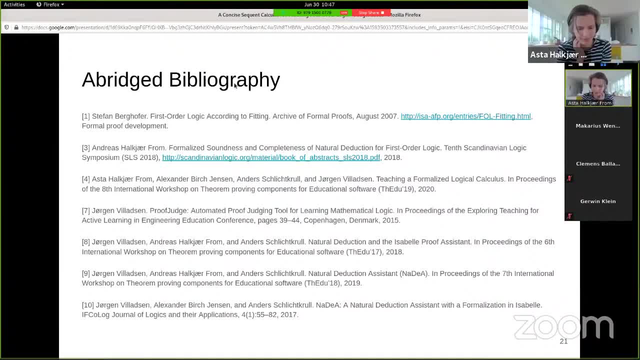 training sessions. some experienced Zoom user pointed out that people are too shy asking on this medium. I have a question. comment You: you said that very early in your talk about your natural deduction system that it would only suggest rules that are actually legal to apply. 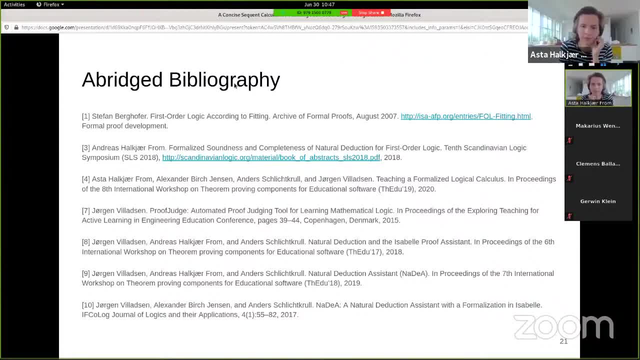 Is that necessarily pedagogically the best thing to do? I mean, I would say that in the beginning, for my students it's not obvious at all when they look at natural deduction which role to apply. So even finding that would be a challenge for them, and so it shouldn't necessarily. 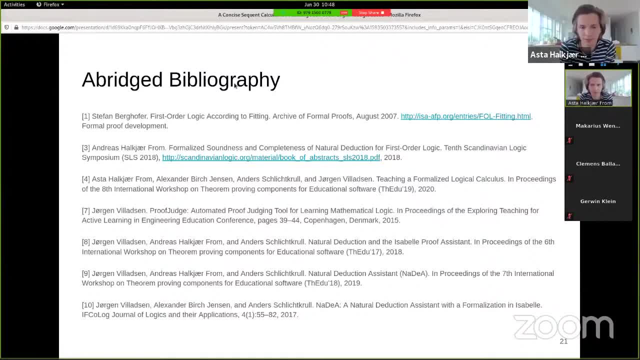 be offered for free, And I mean it's definitely a choice And I agree that there's. there's also an advantage in not making this this addiction for them. Have you ever thought about changing your tools so that you can fine tune how much assistance? 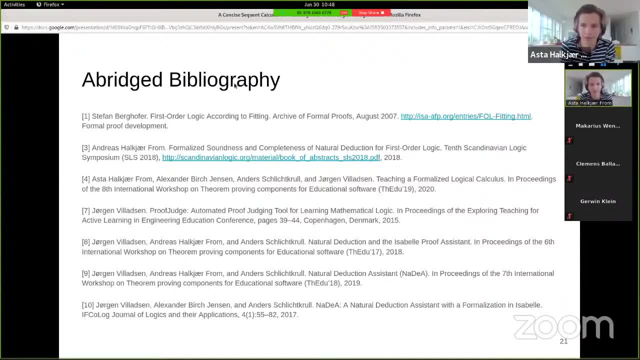 you want to provide to your students The this. so this tool predates me, So I've mostly worked on the formalization. But but yeah, we, we have, we have, we have thoughts in this direction, Thank you, Thank you. I have a question concerning the Isabelle component. I assume in: 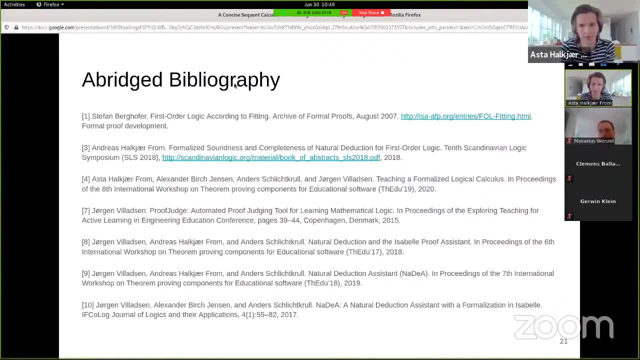 the course the students don't interact with Isabelle at all and they don't really need to understand Isabelle, But it's just that, your front end, that they interact with. For Nadia, I guess for SIG, they work directly in Isabelle And in the course. 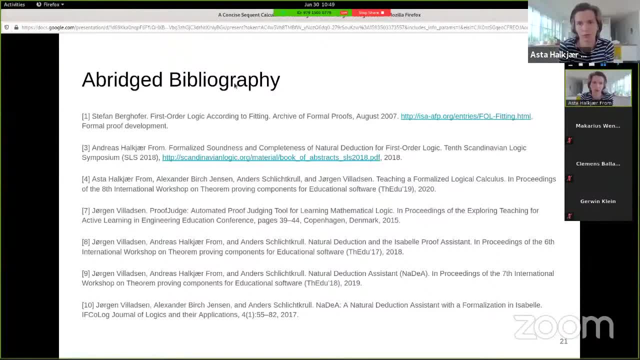 they also worked on a number of other formalizations directly in Isabelle. Sorry, I didn't. I didn't understand this. The students do work with Isabelle, Yes, So for instance, I mean so all the derivations that they do in the Seacom. 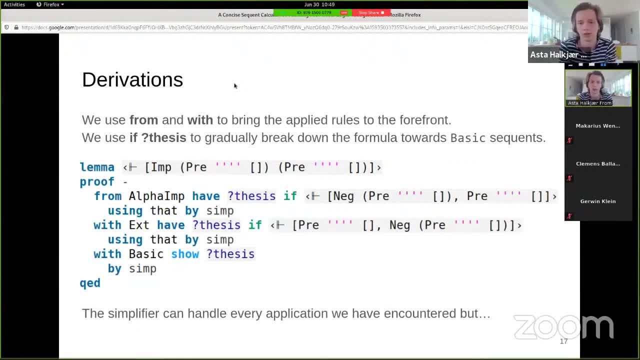 calculus. they do that in the in the J edit. Isabelle editor. Okay, and with the but so you only for Nadia, you have a graphic front end. Yes, exactly Okay, And do you actually find that this helps the students understanding of? 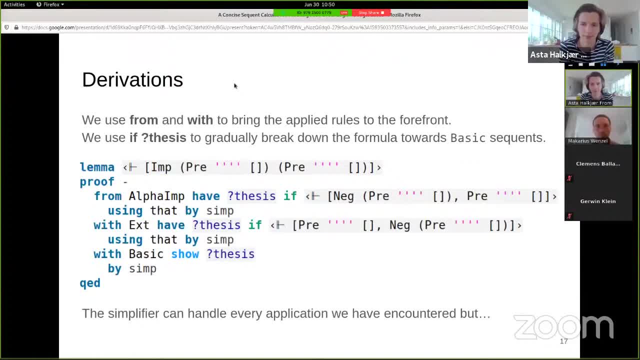 logic that they have to work with these different. Yes, so I think I'm getting echo. maybe I should have one headphones. So a nice thing about Isabelle is that it gives you a warning until you get it absolutely correct. So I think what we saw in the course was that students were actually spending. 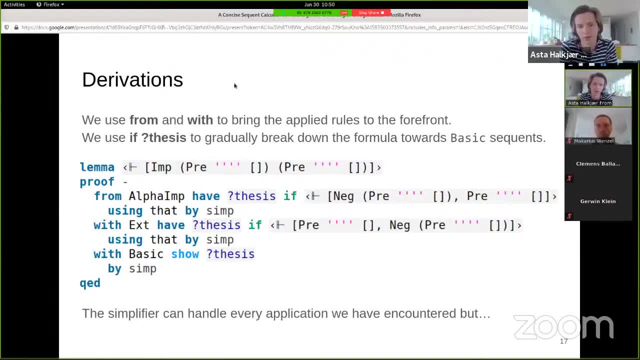 a lot more time working with these proofs than they would have done if they just did them on paper, Because they were. they were like it was like there was a teaching assistant telling them: This is not correct. You can't do this step. 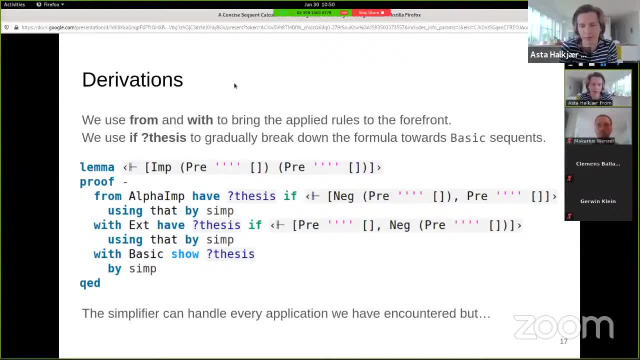 You've got this case whatever, and they they actually worked on it until they got it right. So this may means that the assignments were maybe a little bit harder to create because everyone handed in mostly correct solutions, but I think it also meant that. 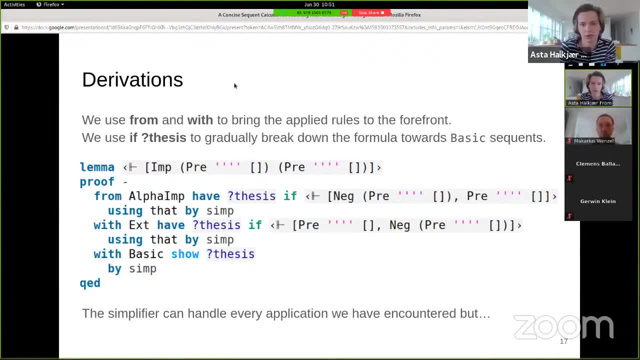 the students put in more work and really worked on it until they they understood all the details. But isn't that the danger that they have to understand a lot more than usually? they don't just have to understand the logic, but they also have to understand the system that realizes this logic, the Isabelle system. 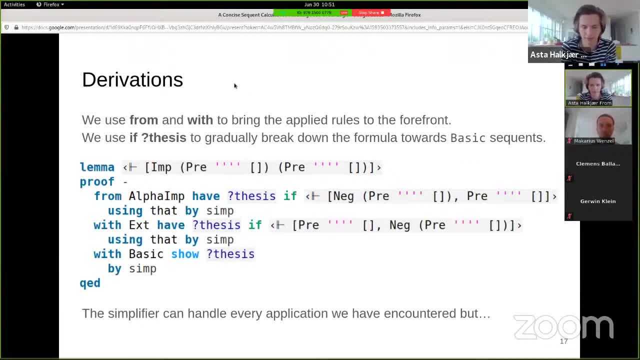 which, to be honest, does have some steep learning curve. Definitely definitely, And I mean so we also. we also introduced Isabelle as just an example of automated reasoning, So it was already something we wanted to do, And then we provide- I mean, we provide- this template for writing these. 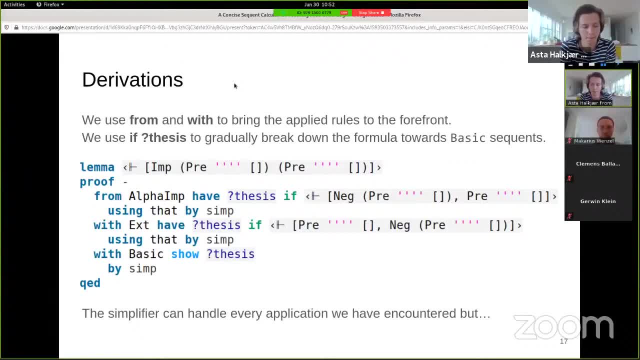 derivations. that seems to cut down on the number of things the students need to understand. Okay, thank you. So you said that you don't have negation in the syntax of the logic you have in Nadia. What is the reason for that? 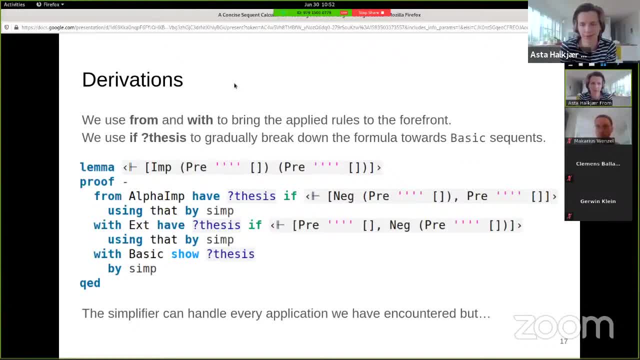 So that's actually a good question And maybe you can answer it, But I don't know if you want to do that. Yeah, I don't know. The Nadia also predates me, So I see Another question: Do you provide some example problems for the students in that web interface? 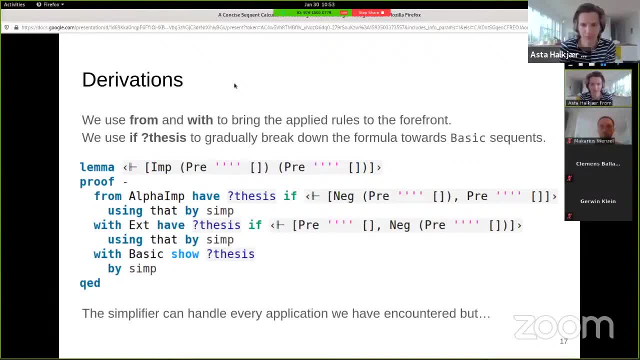 Or have you actually thought about randomly generating formulas that are valid, for which proofs exist just as exercises, Because in my experience, students are always keen on having a lot of examples to work with. I think that would be a cool thing. So in the online application there are: 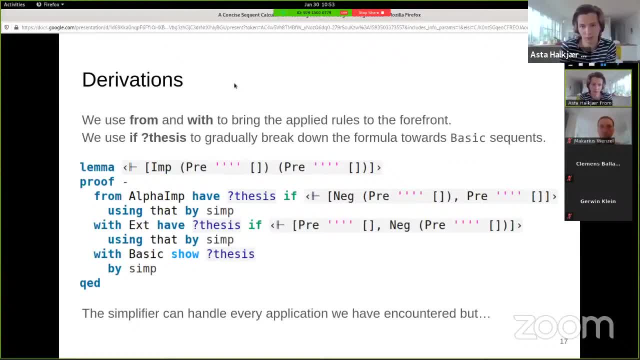 10 examples that you can load of increasing difficulties And there are also 10 formulas that we suggest you can work on And there are some hints available how to get started. But you haven't thought about randomly generating. No, Okay, Thanks. 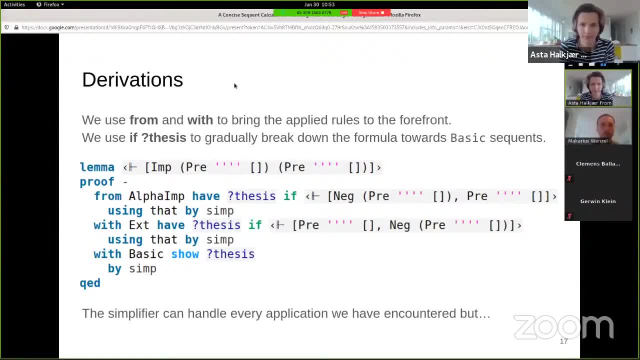 So on this derivation slide you have the cartouche for the inner syntax And then we have to funny single quotes, Therefore string syntax inside H or L. So you consistently using cartouche, I suppose, And would you say that we should do this by default and then reform the string? 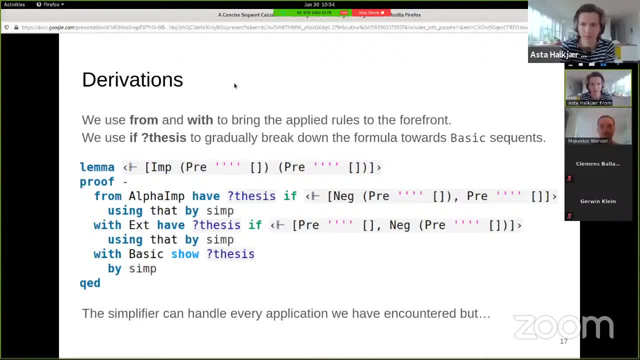 Syntax of H or L to have normal double quotes. Oh so, if you ask me personally, I think yes, I think that would be nice, And you do this consistently yourself- that you always use cartouche. I always use cartouche. 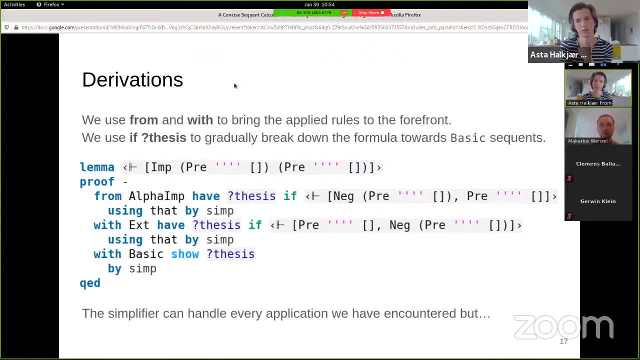 And the students also understood that, how to type it, I mean. so that was a little bit of confusion of how to how to enter them. That's also this. So the way I enter them is is the double quotation and then I press tab.